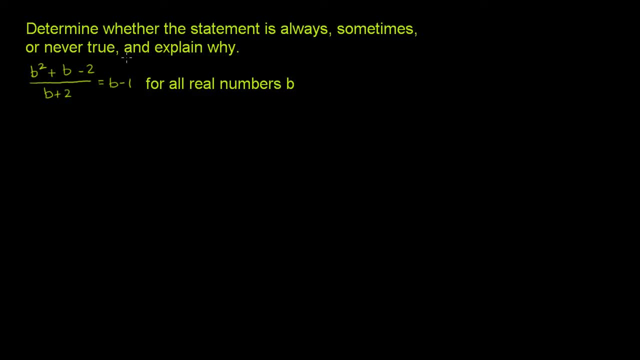 Determine whether the statement is always, sometimes or never true and explain why. The statement here is b squared plus b minus 2, all of that over b plus 2, is equal to b minus 1 for all real numbers b. 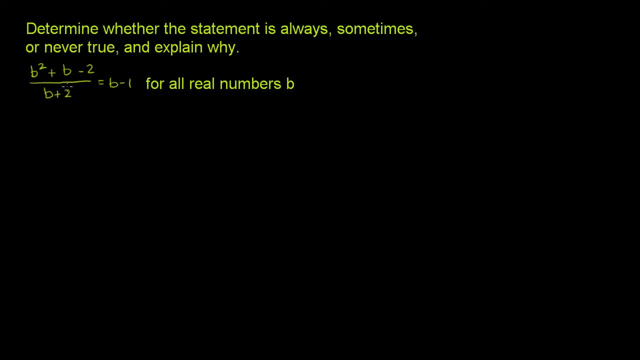 Well, one thing that just jumps out at you, before you even try to manipulate this algebraically, is that I can think of a b value that, where this left expression won't be equal to b minus 1, a b value that will make this left. 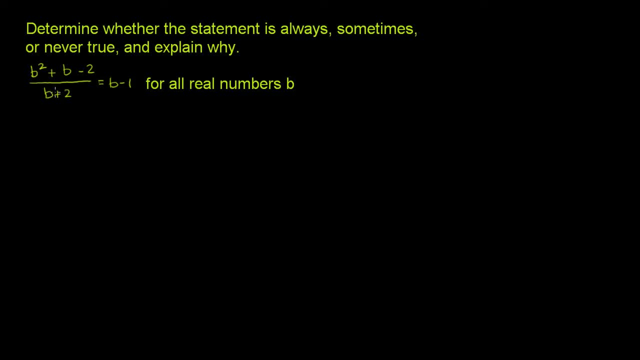 expression undefined. And it becomes undefined if this denominator becomes 0.. And the way the denominator is going to become 0 is if b is negative 2.. So let's write that down: If b is equal to negative 2, then b squared plus b minus 2. 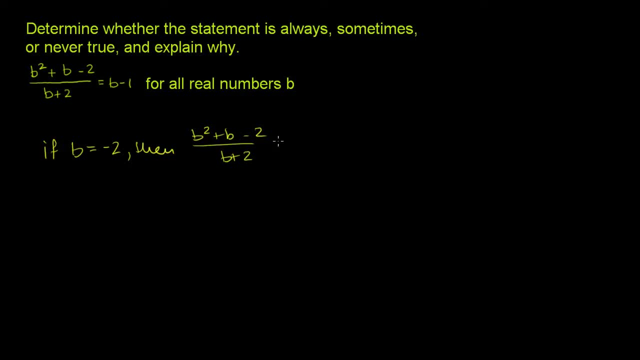 over b plus 2, what does that become? It equals b. squared would be 4 minus 2 minus 2, which would be 0 over 0. Which Is undefined, not, it's not equal to. let me write this: 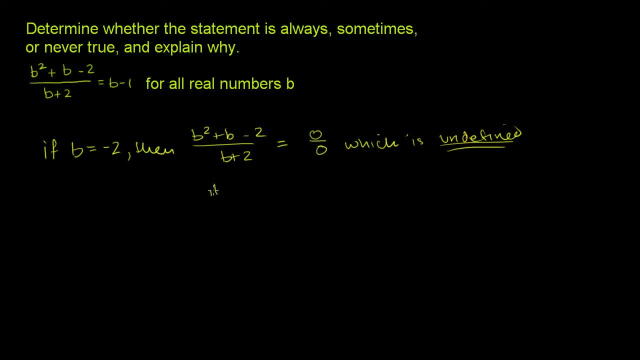 this way it's not equal to. it's not equal to b minus 1, which is negative. 2 minus 1, negative 3.. When you put negative 2 in here, you don't on the left hand side, you don't get, it, doesn't evaluate to negative. 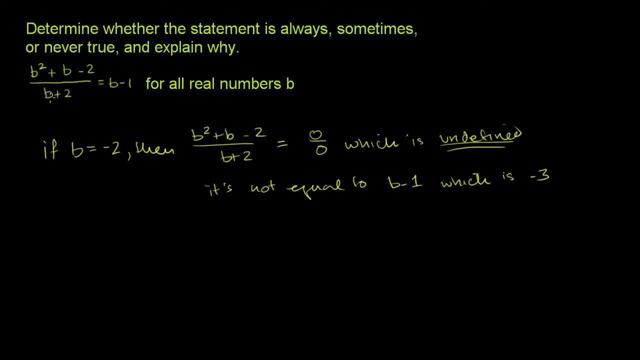 3, it evaluates to 0 over 0, which is undefined. So we already found an example of a, b where this is not true. So it's definitely not always going to be true. We found a case. Now let's algebraically manipulate this and see if 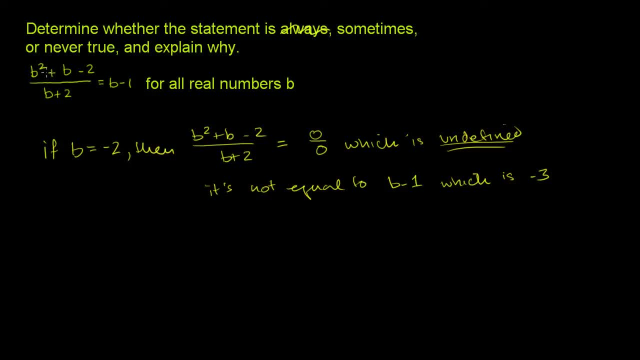 it's true for pretty much any other number. So let's see if we can maybe factor the numerator up there, So b squared plus b minus 2, if you think about it, a number- that two numbers when you take their product- is negative 2,. 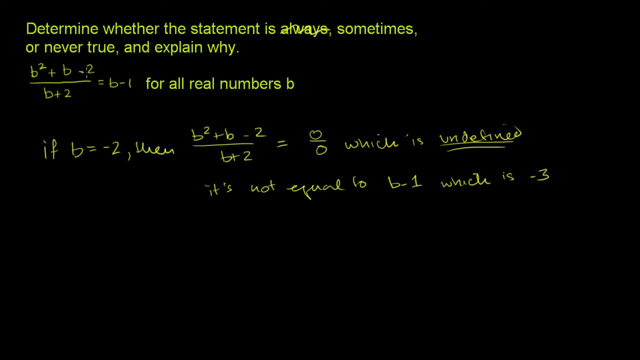 and when you add them you get 1,. well, that's going to be positive 2 and negative 1.. So the numerator we can rewrite as b plus 2 times b minus 1, and then the denominator is b plus 2, and then, well, we.